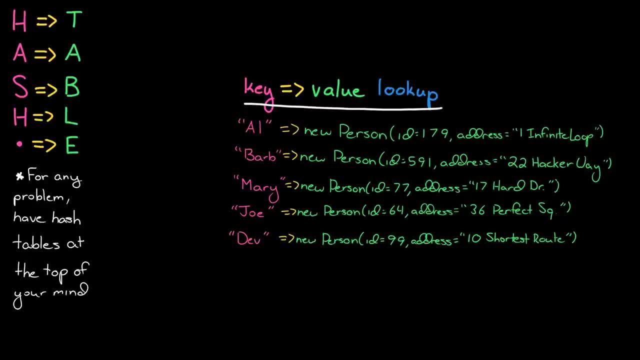 associating a value with it for very, very quick lookups. So suppose you had some situation where you needed to associate somebody's name with some set of information about them. A hash table would be the perfect solution for this problem, because you can just put this into the hash table and then. 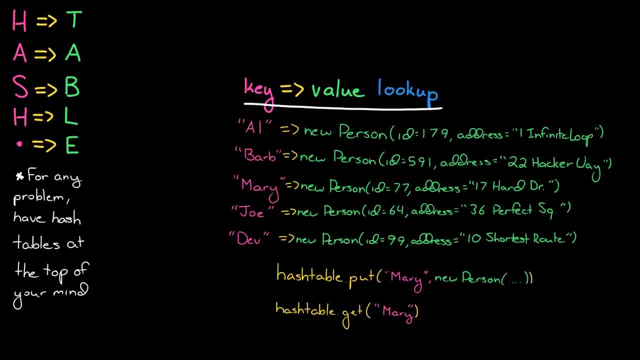 you can say: okay, give me the data associated with Mary, and then boom, you can get that information immediately. So you can just put this into the hash table, and then you can say So. in a hash table, the key, as well as the value, can be basically any type of data structure. 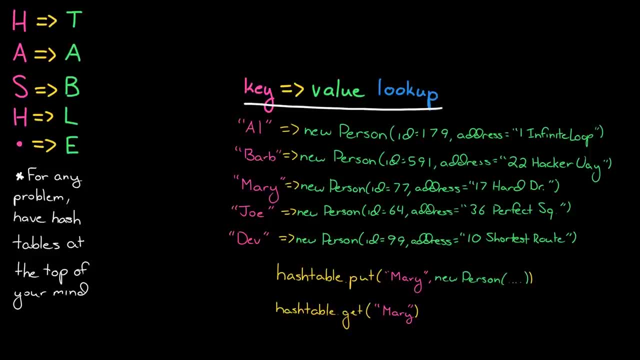 A string is often used, but it could be a circle, a square, a person, pretty much anything, as long as you have a hash function. So what does that mean? Well, let's turn to the implementation to talk about that. So, at a high level, we do want to store the objects in an array. So let's picture: 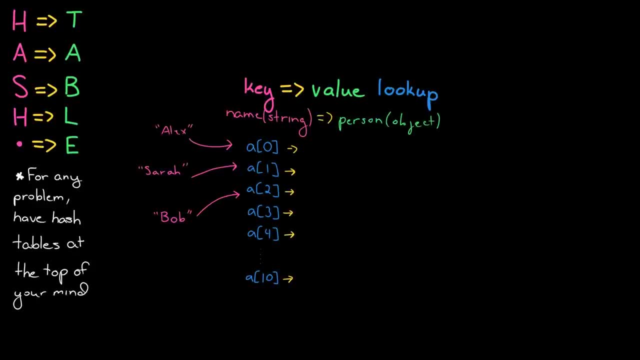 that. But how do we actually jump from a string to a particular index in the array? Well, that's what a hash table does. It's a way of storing the objects in an array. So let's picture that. So a hash function takes in a string, converts it to some sort of integer and then remaps that. 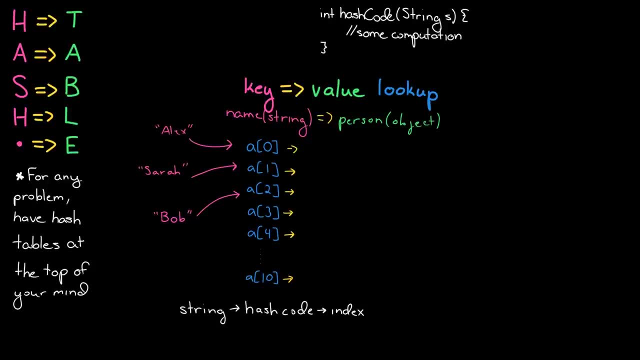 integer into an index, into that array, And then that's where we can find the person we're looking for. So it's important to understand that the hash code is not actually the index in this array. We map actually from the key to the hash code and then over to the index, And one of the reasons for 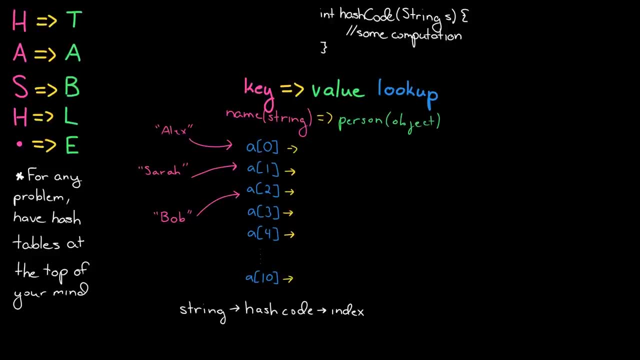 this is that the array that actually stores the data from the hash table might be much, much smaller than all the available potential hash codes, And so we don't want to have an array of three billion just because there's three billion potential hash codes. So we actually 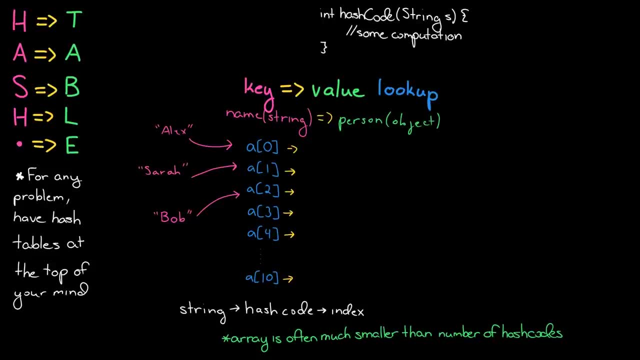 remap it into something smaller. Now note here that two different strings could actually have the same hash code, And that's because there are an infinite number of strings out there but a finite number of hash codes. So it's theoretically possible for Alex and Sarah to 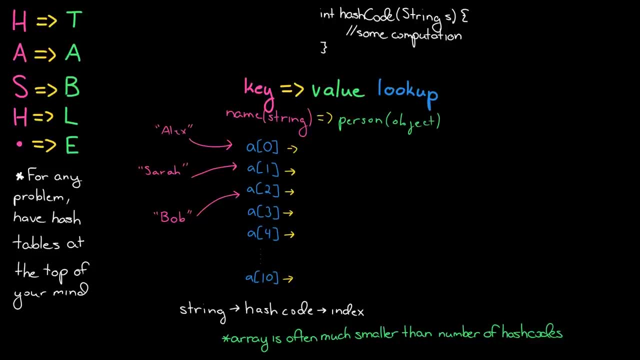 actually have the same hash code. Additionally, since we're remapping the hash code, we're going to be remapping the hash code into an even smaller index. Two things with different hash codes could actually wind up mapped to the same index. So what do we do with this? when this happens, which is: 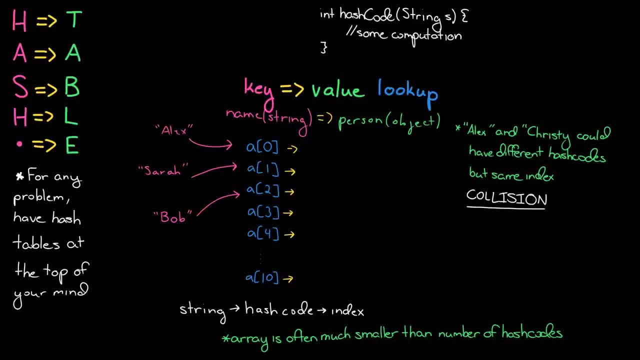 called the collision. There are different ways of resolving collisions And I really do encourage you to look this up on your own time, But I'll just talk about one of them, which is called chaining, And chaining is possibly the most common one, And it's very simple What it basically means. 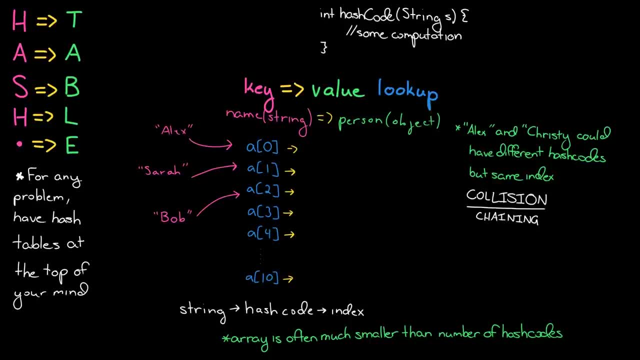 is just: hey, when there's collisions, just store them in a linked list. So, rather than this being an array of people, it's actually going to be an array of a linked list of people, And so that means, though, that when you get a call to say, hey, get the value of Alex, you actually need to look. 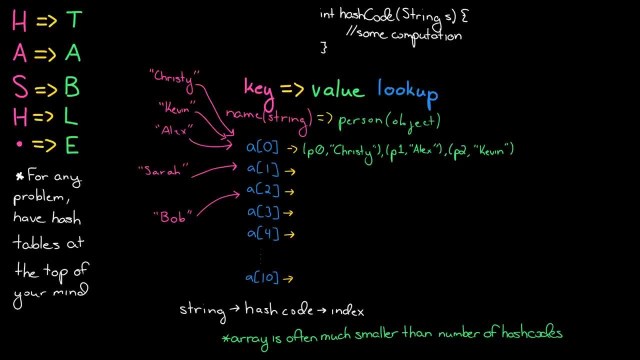 through all the values in that linked list and pull out the value for Alex. Now, as you'll note here, this linked list contains not just the actual person objects but the actual original keys as well, And the reason for that is that if you only store the person object, 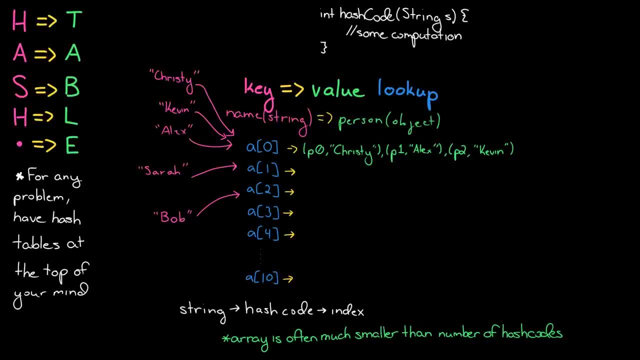 you'd see all these people who map to this index, but you wouldn't know which one they are, And so you actually need to store the keys with them. So when you get a call to say, get me the value for Alex, then you actually call this hash function. you get a hash code back. 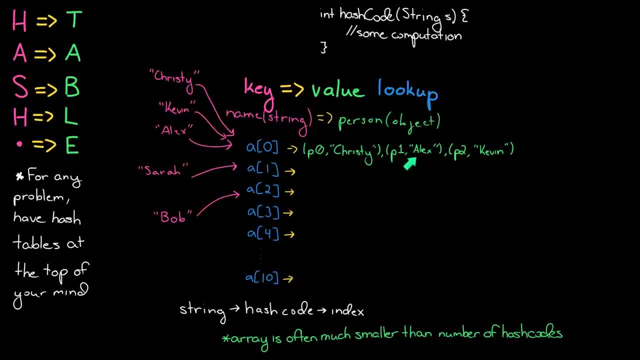 you map over to this index and then you walk through and look for the thing with the key of Alex. So that's the basics of how a hash table operates. So let's walk through this from start to end. We're going to have this hash table class that, underneath it, has 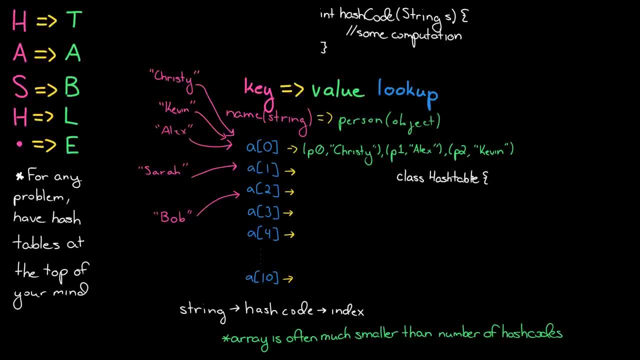 an array that actually holds the data, And the array isn't going to be an array of the actual values, It's going to be an array of the linked list of the values. Then, when someone says, put the value of Alex, put the value of Alex mapping to this person. 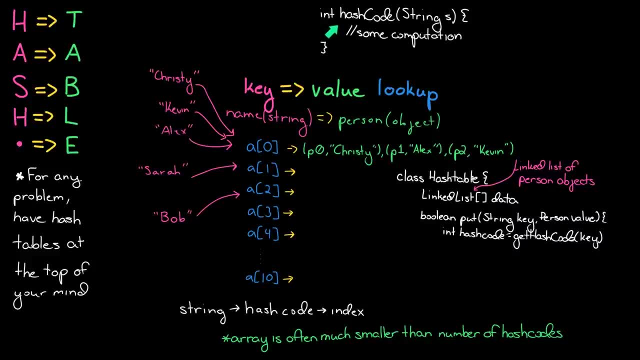 we call this hash code function. that gets us back the hash code, Then we map from this hash code over to an index and that gets us over to this index in the array And then we put it into the linked list. If there's nothing else great, Then we're just going to have a one element linked. 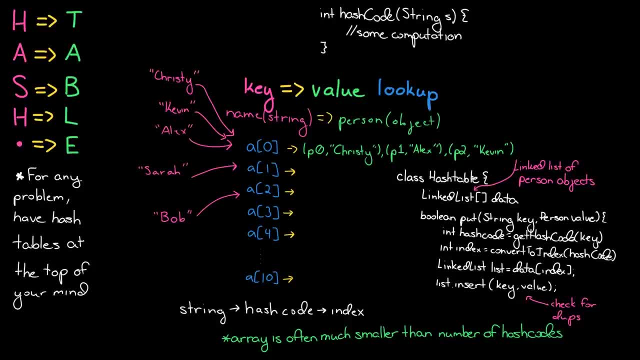 list, But there could be multiple values in there, in which case we walk through it. Now, what if there are already a value of Alex in there? Well then, we just fix that value immediately. So let's talk now about the runtime of a hash table. Well, it really depends on what we're. 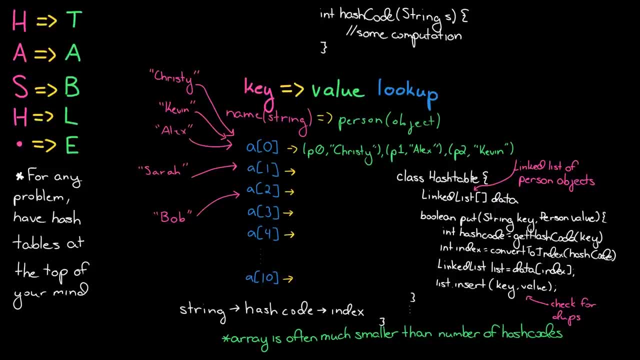 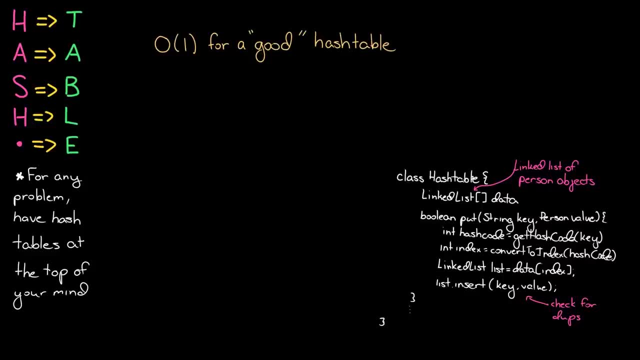 talking about and what assumptions we make. In many cases we assume that we have a good hash table and a good hash function that we're going to be able to use, But in many cases we assume that really distributes our values well, And so for the purpose of an interview, we often just